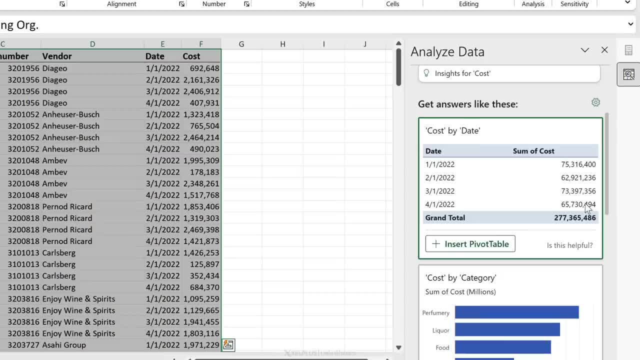 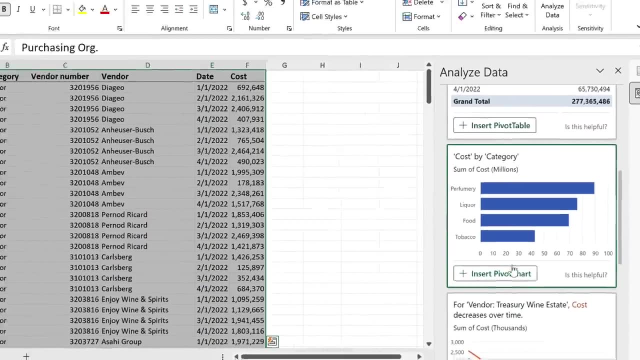 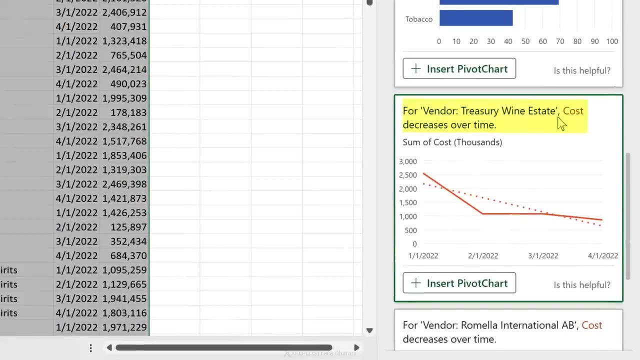 and the sum of costs. My numbers also look like they have perfect formatting Down. here I get cost by category. I could just insert this pivot chart and it's going to insert it on a separate sheet. Here I have some additional insights. So for vendor: treasury wine estate. 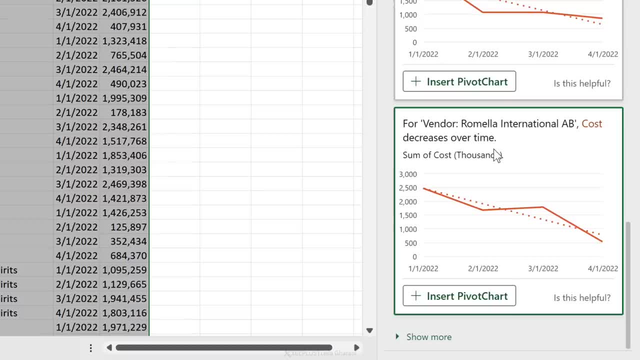 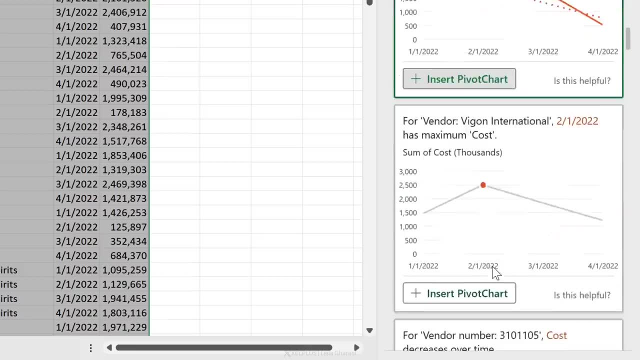 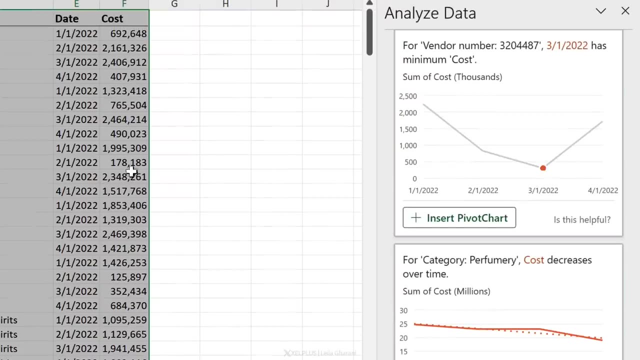 cost decreases over time. Well, this could be interesting for my boss. I wasn't specifically looking for this. Also for this vendor, cost decreases over time. I can go to show more and get my data, Maybe find out something that is going to surprise me and something that I might need to. 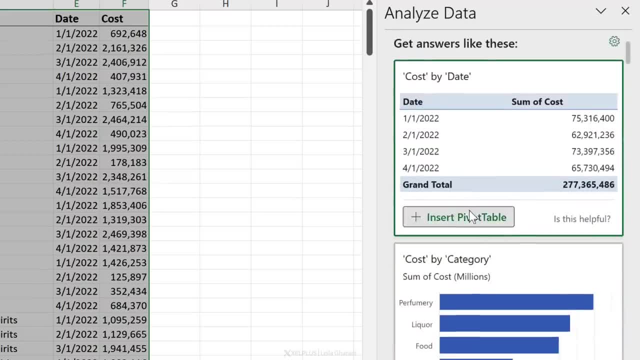 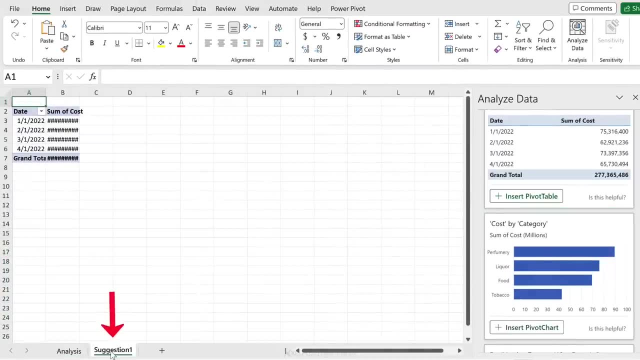 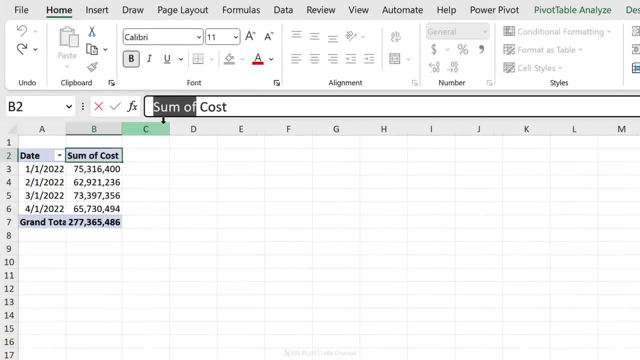 follow up on, But right now I don't need to worry about this, because my boss asked for a summary. This is a good summary to have, So let's insert a pivot table and see what we get. We got a new tab date and sum of cost, So I'm going to change that to be total cost Now. 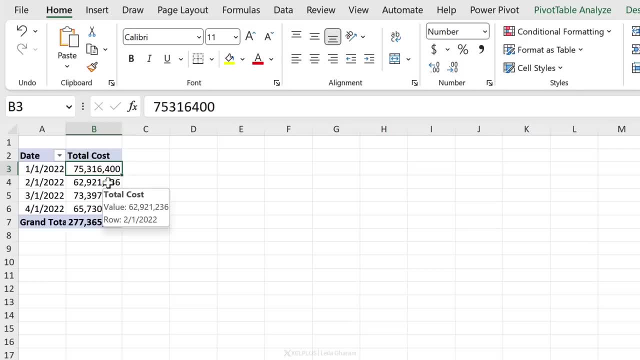 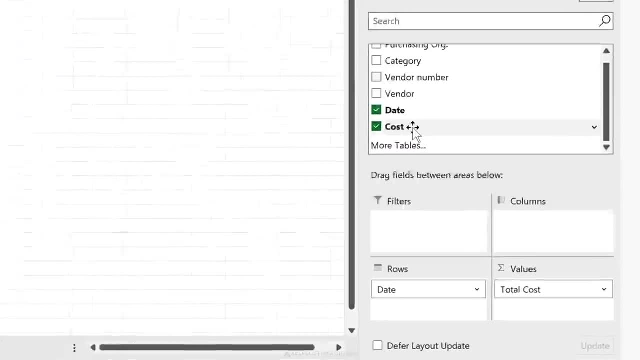 I also know that my boss is interested to find out what the average cost is, Since I already have my pivot table and I have my layout right here. it's quite easy to do that. All I have to do is grab cost and drag and drop it in the values. So I have it two times here And for the second time. 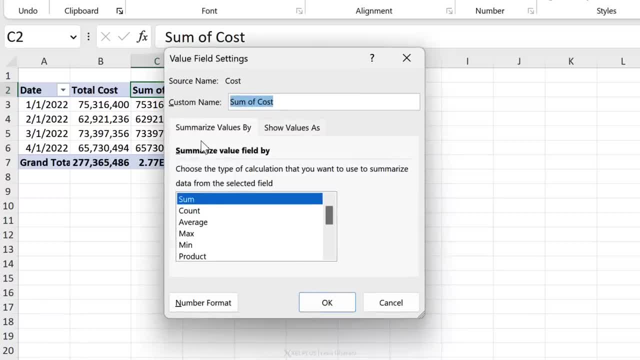 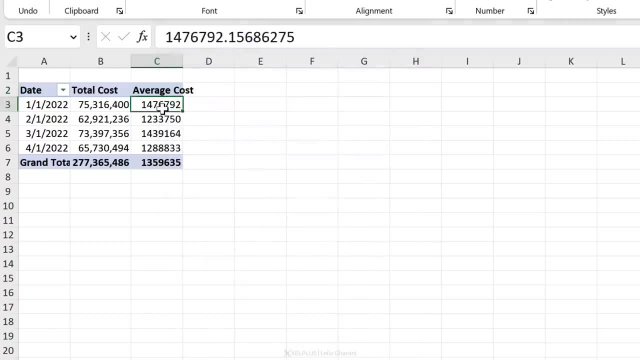 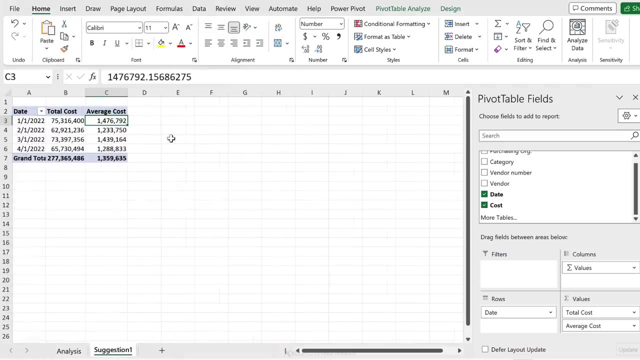 I want it to show the average values. I'm just going to double click, go to average, change this to average cost and click on OK. All I have to do is update the formatting. Right mouse click number. format number: use a thousand separator And that's it. We're done. Now, what about that? 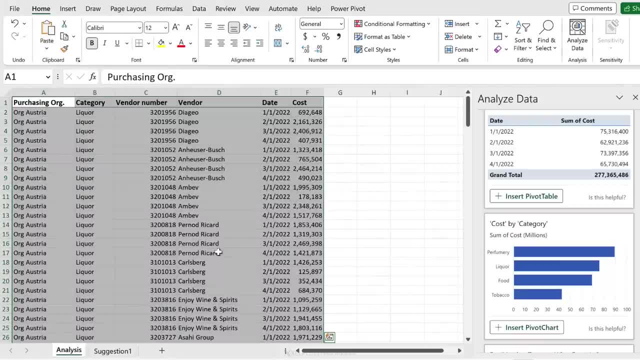 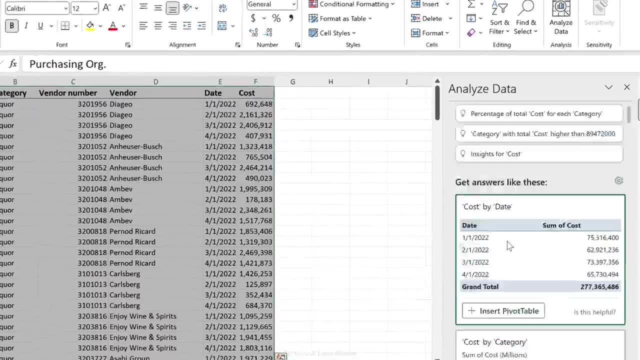 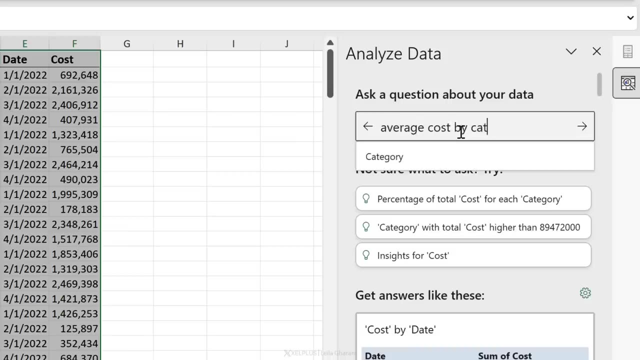 chart. That was interesting as well because we want to take a look at the cost by category. So that's the one I want, but I'd like it to be the average cost per category. So let's see if we can ask it to specifically create that chart for us, Average cost by category. I think that should. 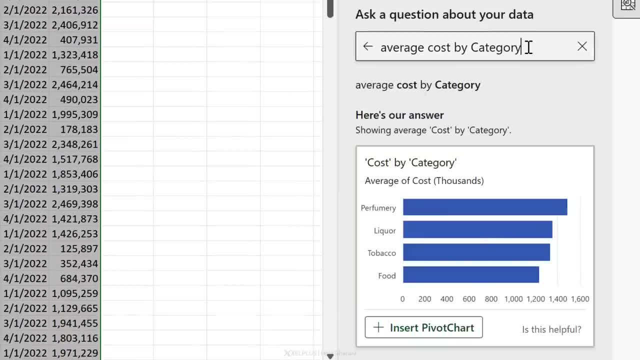 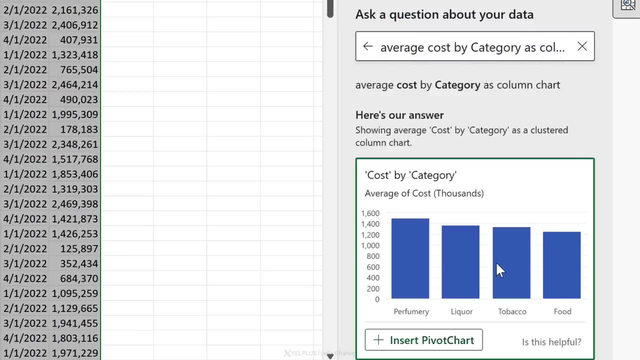 do. Yeah, we get our pivot chart. Now, what if I wanted it as another chart type? So what if I said: as column chart, Does that work? Yeah, that works as well. So this is better. Let me just insert it. I get a new tab with a pivot table. That's. 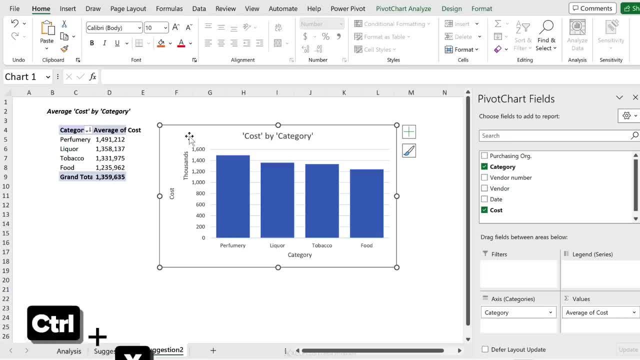 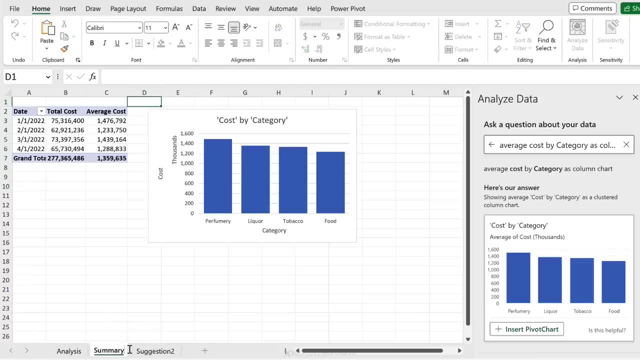 the underlying data for my chart. I'm just going to cut this and paste it here. So this, ultimately, is going to be my summary sheet. This is going to be my underlying data, So I'm just going to keep it somewhere. I'll probably hide this in the end. Let's quickly. 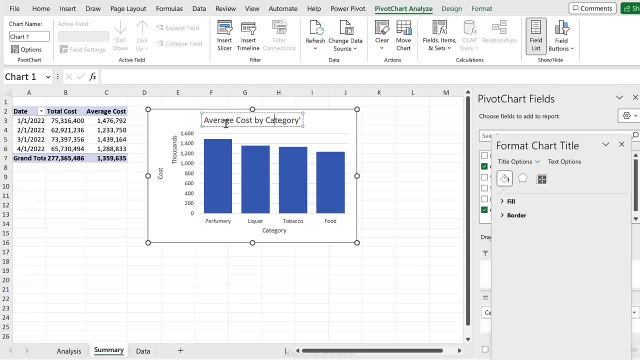 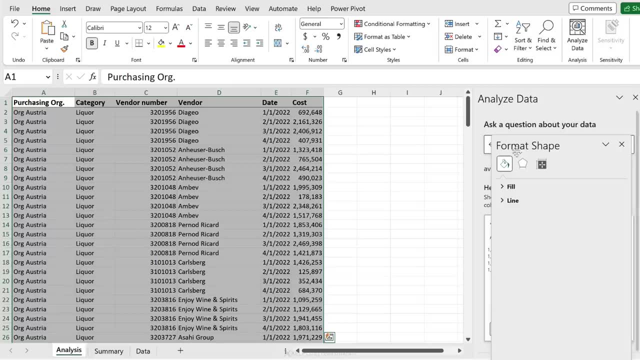 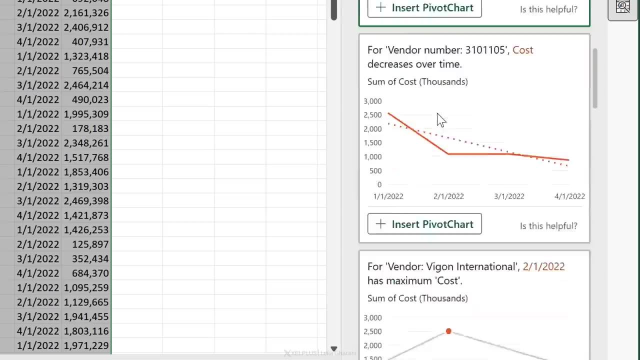 just update this, So it's clear that this is the average cost by category. Now what if you also want a line chart here? Let's go back. Let's just type in cost trend, Let's see if it understands. Well, it's giving me some specific things: Cost over months. Yeah, that's better. That's what I. 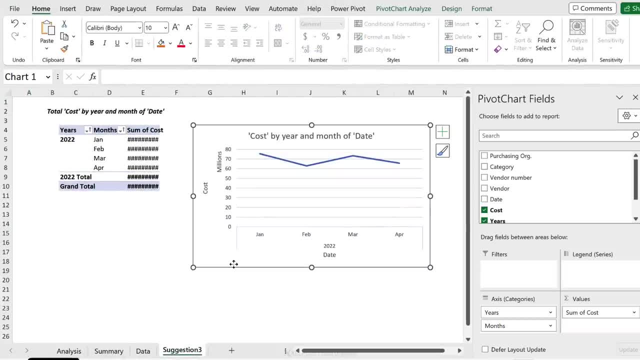 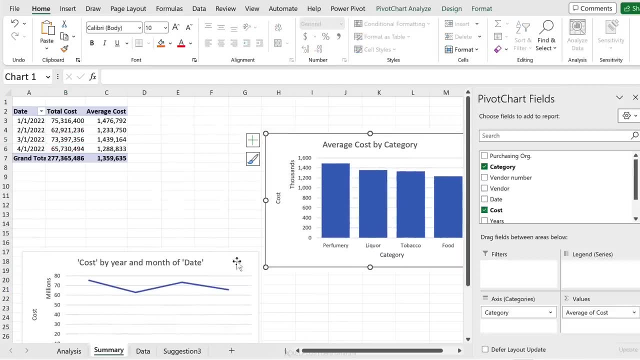 want. So let's go and insert the pivot chart as well, And we could grab that and bring it over to our summary sheet, right? So you'll have to format these accordingly if you need to. Let me also quickly clean this up a little bit. So let's go back to our summary sheet. Let me also 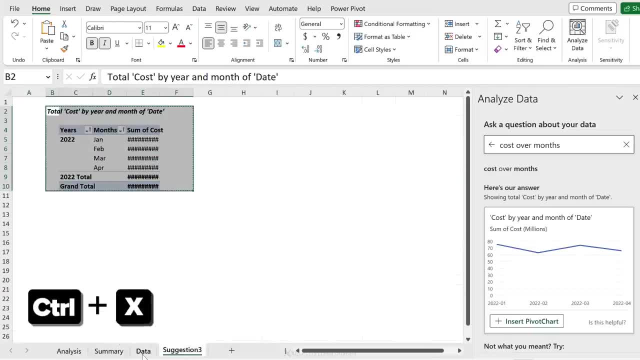 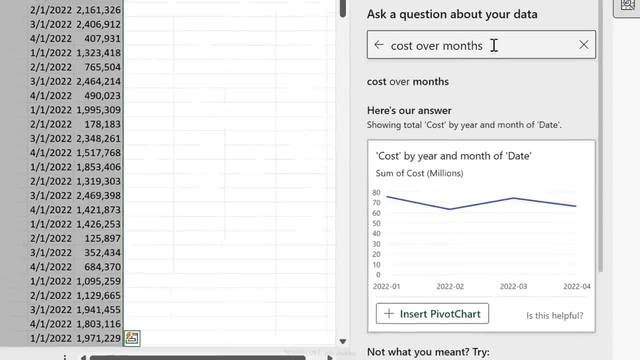 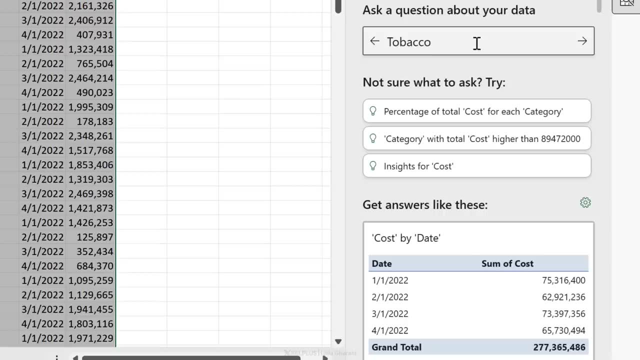 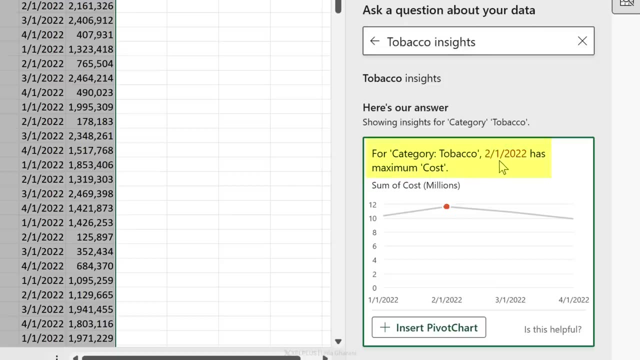 Now, what about specific insights? So if we go back here, let's take a look at tobacco. So I'm just going to type in tobacco- It's actually easier to pick it from here than to type it in- And let's go with insights. Okay, So for category tobacco, February had maximum cost. 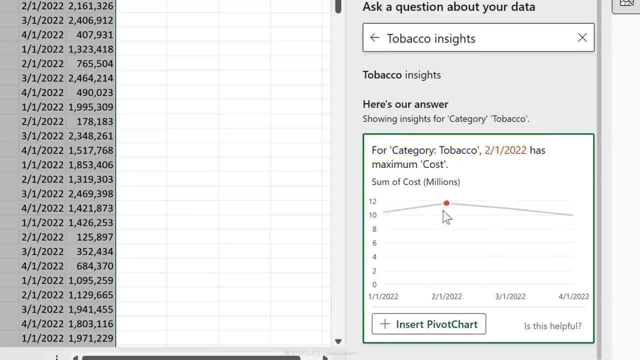 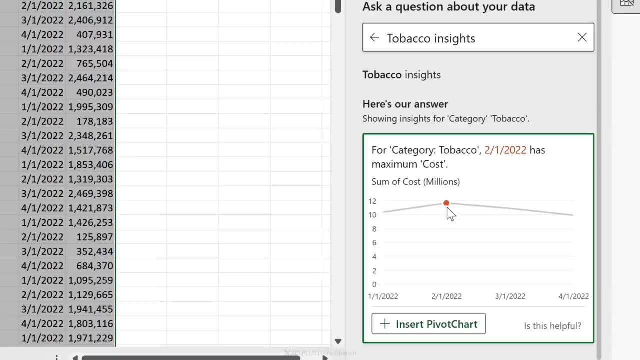 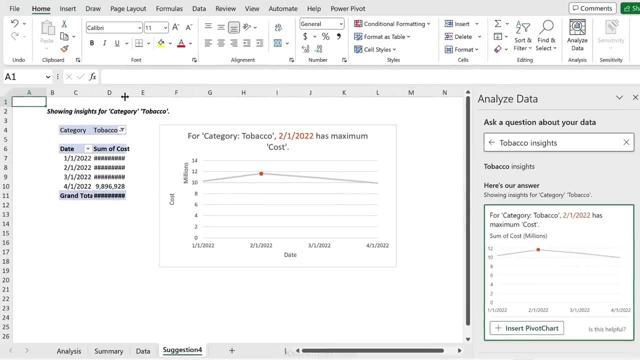 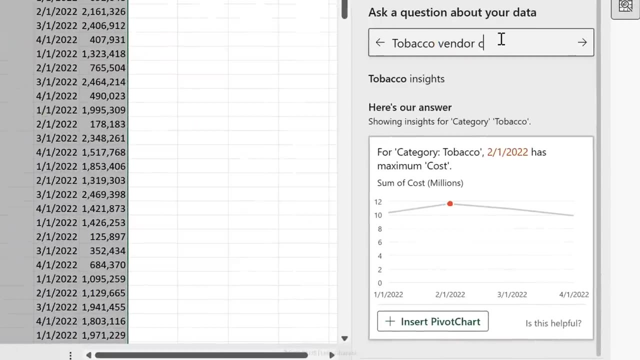 conditionally formatted it by highlighting the maximum point. here, All I have to do is insert the pivot chart and I have it right here. What about if we wanted the vendors as well? So let's go and see tobacco vendor cost breakdown. Okay, I spelled that wrong, but it's still got it and it looks. 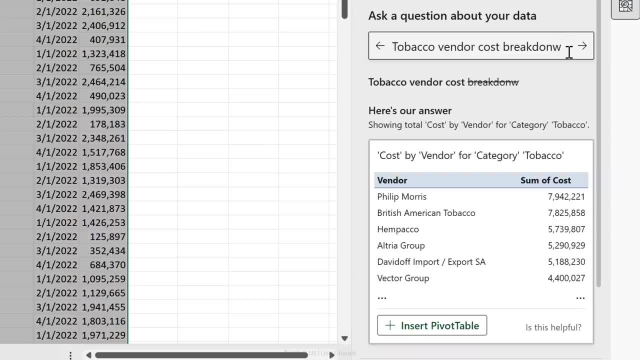 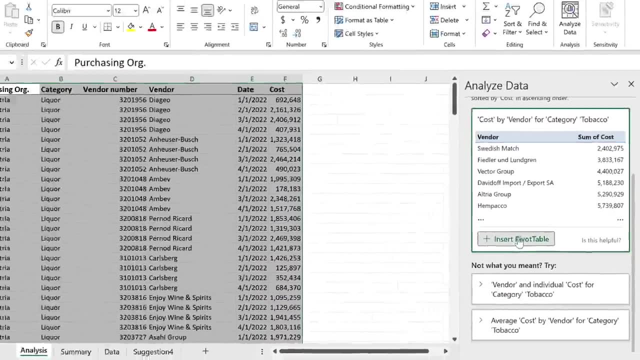 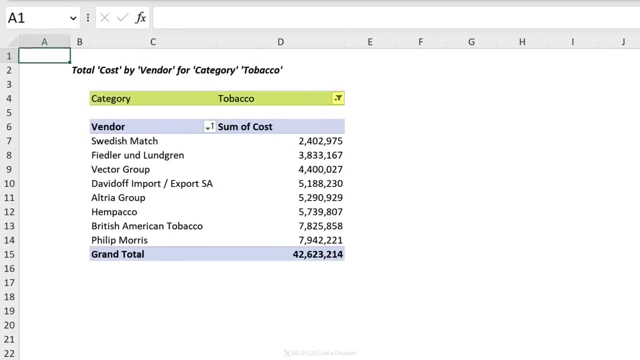 What if I wanted to sort it the other way around? Let's do sorted ascending. That works as well. Okay, Let's insert a pivot table, And here's our report. The category tobacco was already added as a filter to our pivot table. 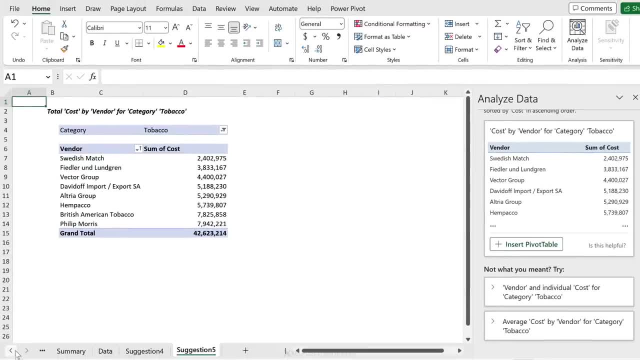 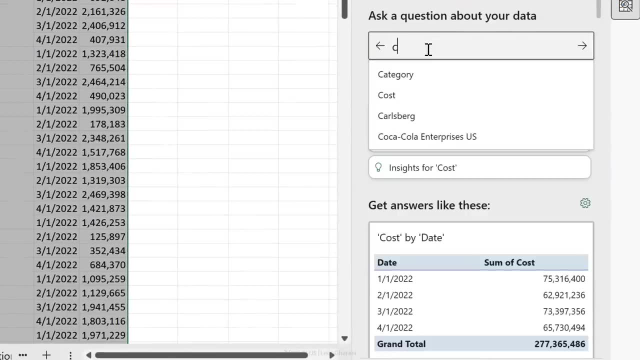 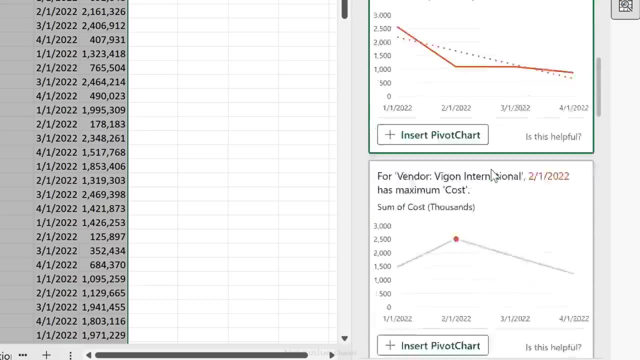 How great is that? Now, what about some specific insights? So let's go back and ask for cost insights. Actually, we see it right here, So let's just select that: Insights for cost. That's what we saw before as well, So let's just add some of these. I even get frequency of cost. 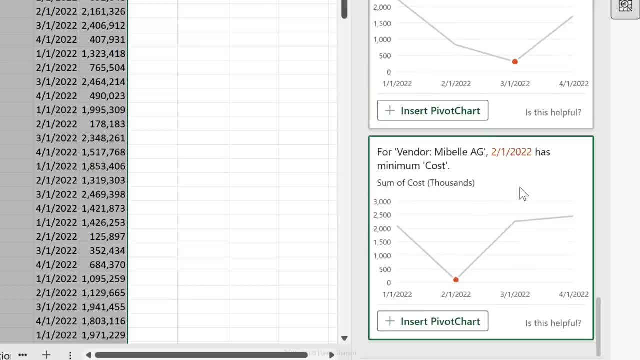 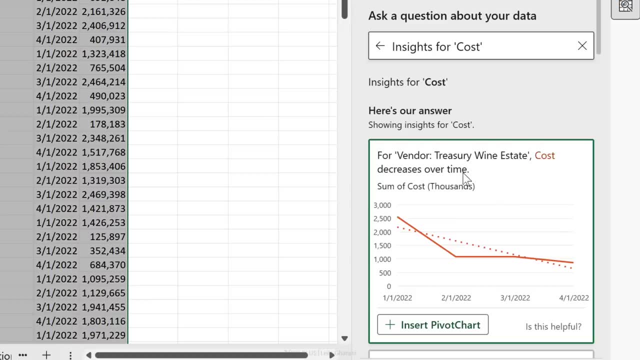 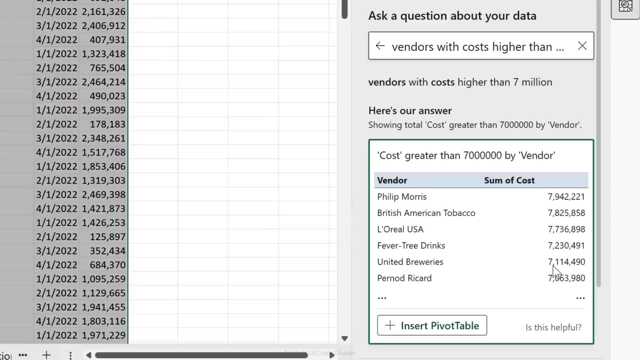 Okay, This one is interesting. This is interesting as well. What if I wanted to see the vendors that have a cost above a certain threshold- Let's see if we can get that done- Vendors with costs higher than 7 million. It picked up the 7 million correctly, So all I have to do is insert. 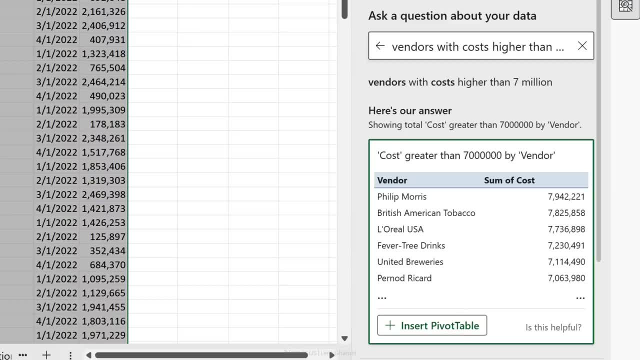 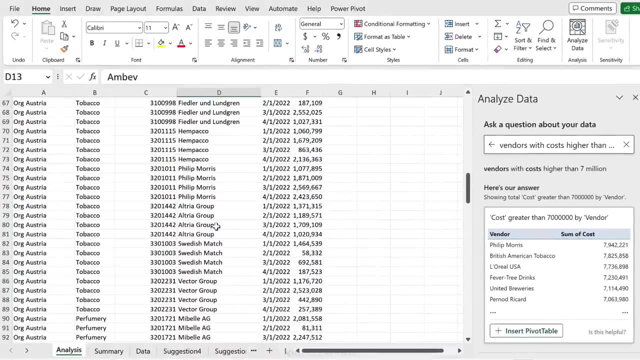 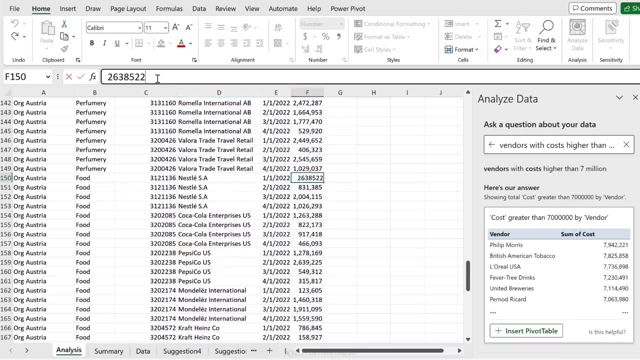 this pivot table and then insert some of the other ones that I got from the insights, and my task is done. Now you might be wondering: are these dynamic? So if my data changes here, is everything going to change? Well, let's try it out. I'm going to go to food here. Let's change one of these. 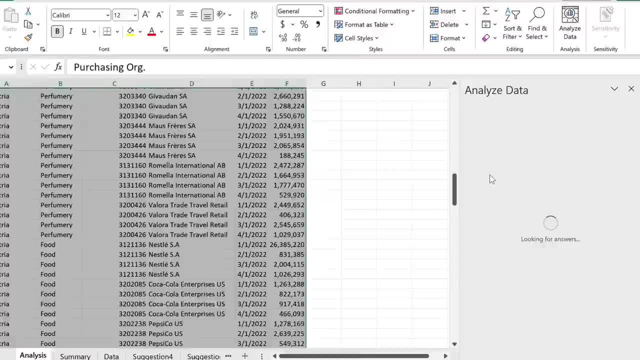 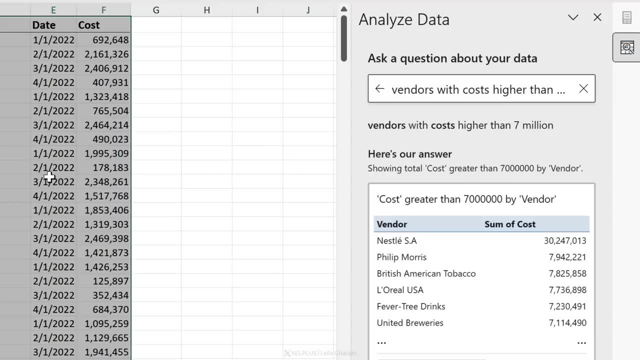 numbers. Let's just add an extra zero, Okay. So here we are. I added a value, I'm changing it to a lot. add an extra zero, okay. so here it tells me it looks like your data is changing and it's reanalyzing my data. so that's great. I don't have to do any specific type of refresh, but if I want, 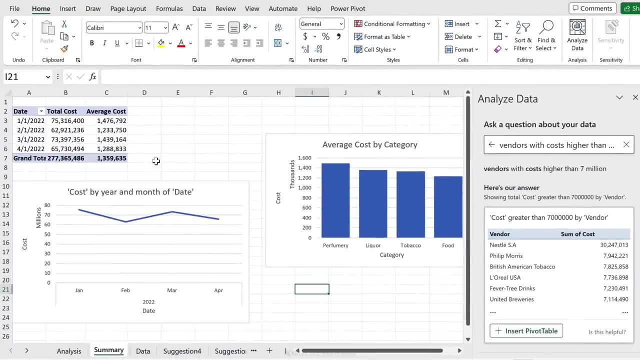 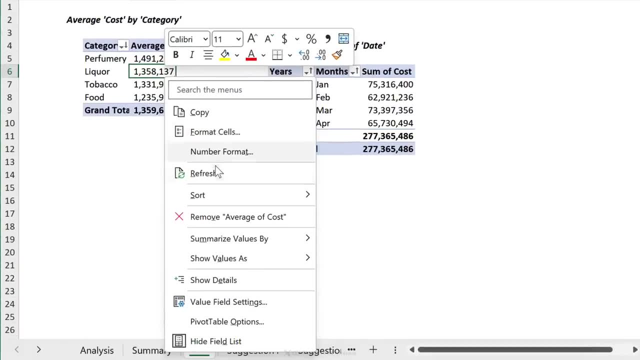 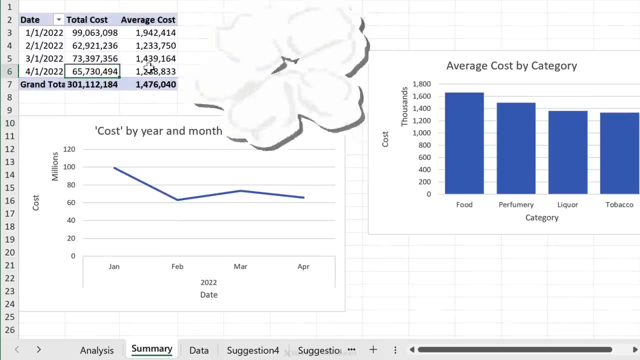 my pivot tables to update as well. I have to do a refresh. so where was that for food? right, if I just update it here, just so that we can visually see it change? I'm going to refresh and this changes, but it's not only this table, it's all the other tables that were created as well, so this one. 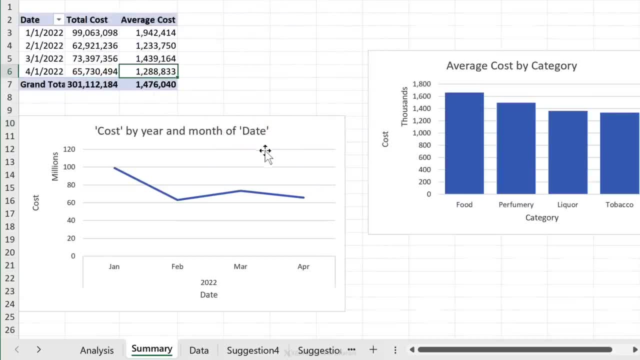 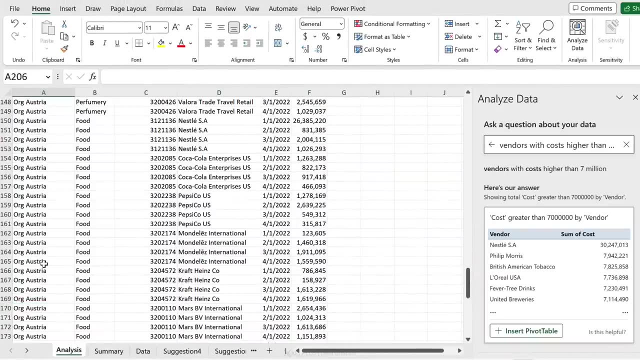 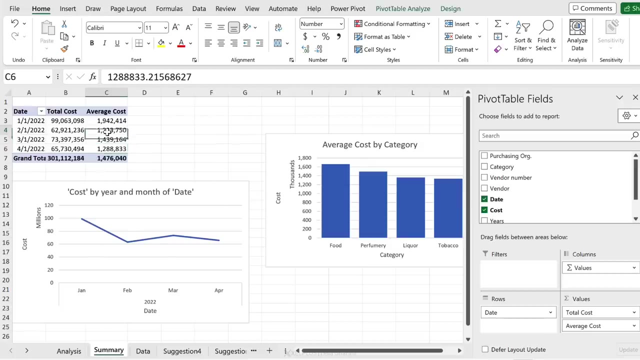 changed as well. so did all my other pivot charts. now, if you want to add data to the bottom of this, it's best if you format your data set here as an official excel table. this way, your pivot tables will automatically update the moment you press refresh and you don't have to update your range. 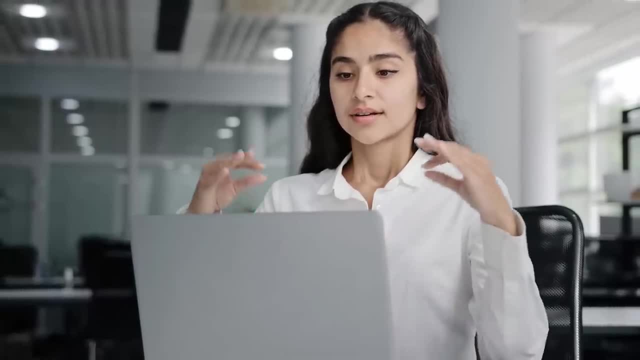 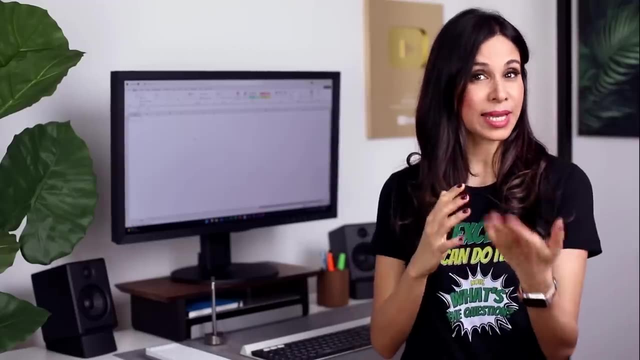 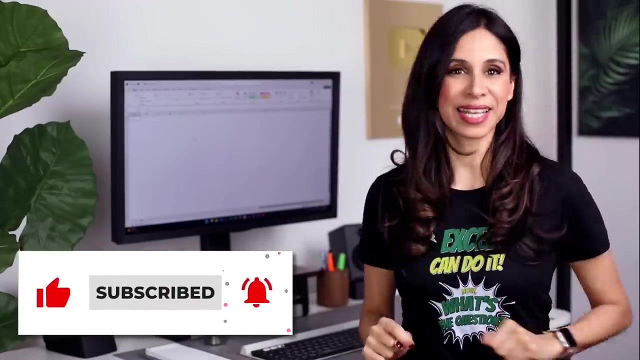 isn't that amazing that with just a few clicks, we get to create a functioning report? all right, so that's one place AI can help us analyze data in excel. use it and let me know what you think. thank you for watching. thank you for being here. subscribe, if you aren't subscribed yet, and I'm going to catch you in the next video. 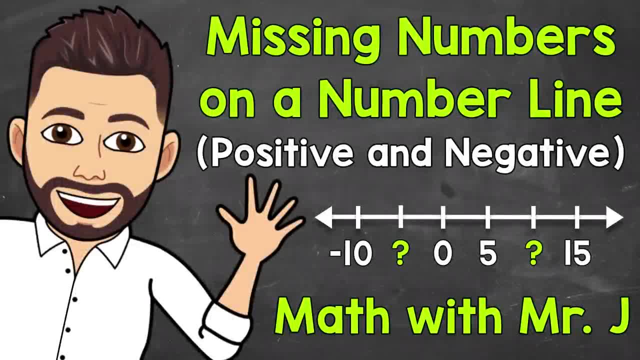 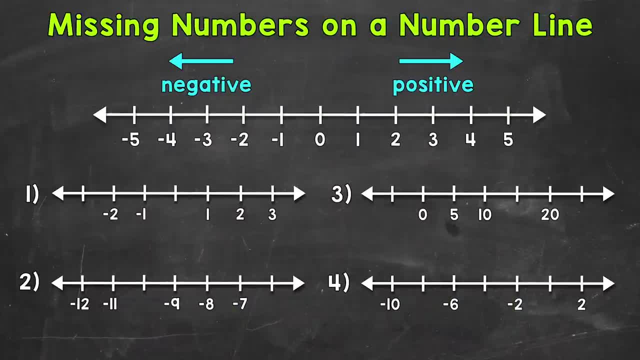 Welcome to Math with Mr J. In this video I'm going to cover how to find missing numbers on a number line. Now remember: to the right of zero we have positive numbers and to the left of zero we have negative numbers. 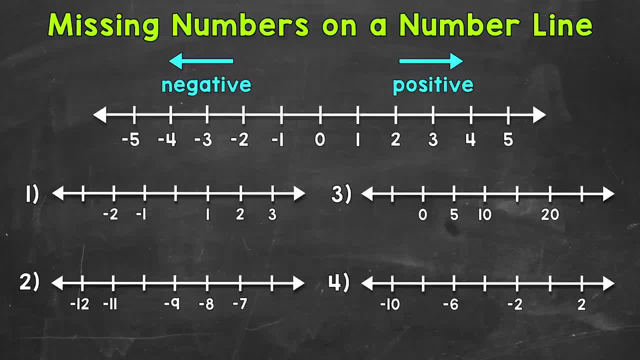 Another thing that I want to mention before getting into our examples, is that when we move to the right on a number line, we increase in value, And when we move to the left on a number line, we decrease in value. So keep that in mind. 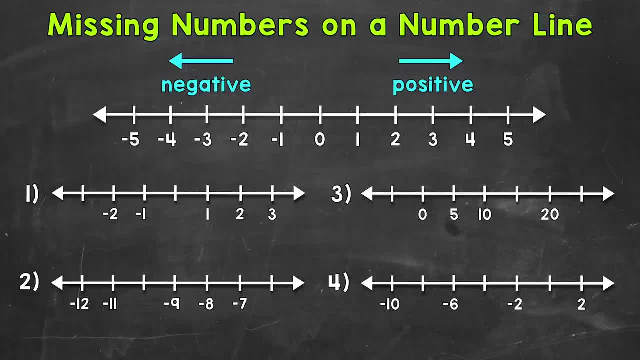 Let's jump into our examples and see exactly how we find missing numbers on a number line, starting with number one. Now, the first thing that we want to do is take a look at what we are given and determine how far apart the numbers are on the number line. 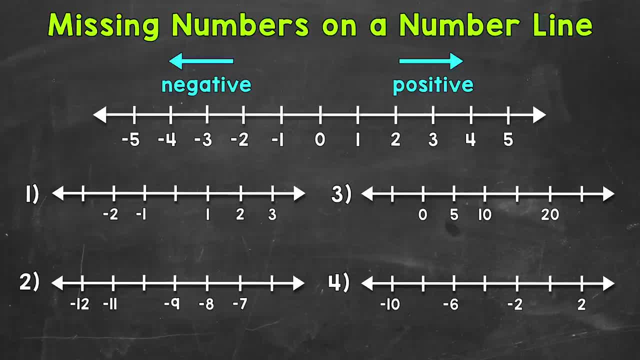 You can think of it as seeing what we're counting by. So we're given negative two and nine, So there's a distance of one between those two numbers. We're also given one, two, three, So the distance between those numbers is one as well. 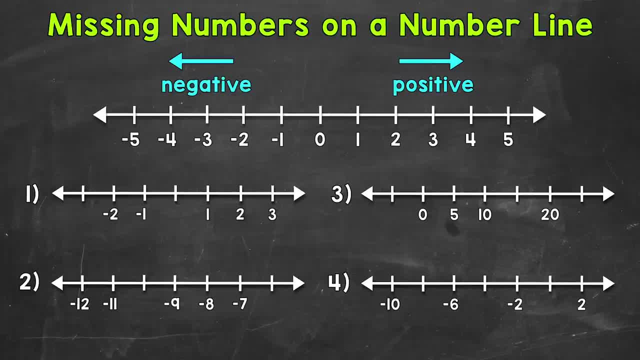 So we can see that we are counting by one. Once we figure that out, we can find the missing numbers. We can either count up or count down using that distance between numbers in order to find the missing numbers. So, for example, let's count down from three.